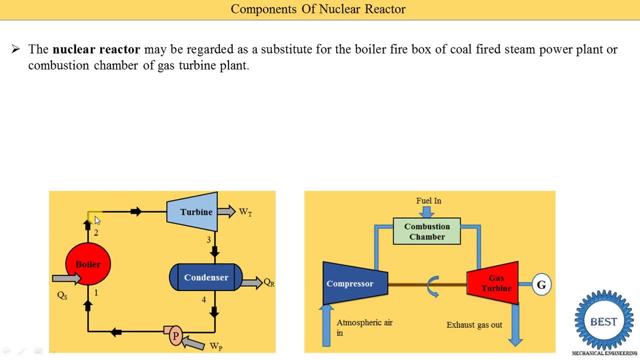 we use the boiler to convert the water into the steam, and in the boiler there is a combustion, of fuel is carried out. Okay, same way. in a gas turbine power plant, we use the combustion chamber to heat the air or a gas coming out from the compressor. So same way in a nuclear nuclear power plant. the nuclear reactor is used to heat the working fluid means working fluids, maybe water or a different types of gas. Okay. so in a 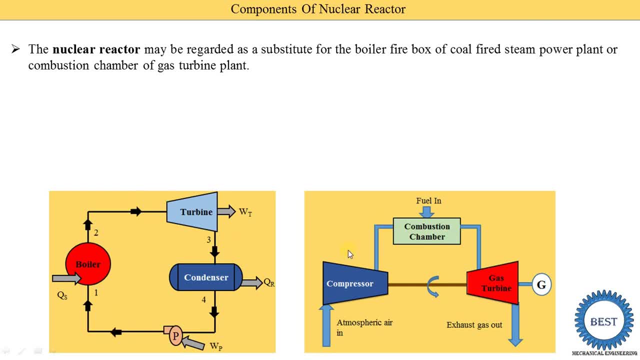 n-kind cycles or a steam power plant, it is fixed the working fluid is the steam. in a gas turbine power plant, it is fixed that the air or gas is used as a working fluids. okay, so in a nuclear reactor we are able to use the steam as well as gas as a working substance. the heat produced in 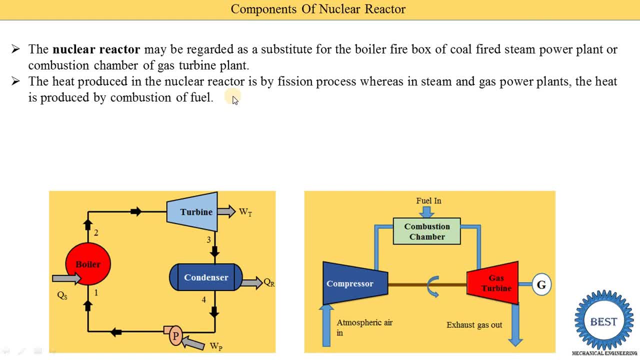 the nuclear reactor is by the fission process. okay, means in a nuclear reactor the process is carried out. it is called as the fission process. in a steam and gas turbine power plant the heat is produced by the combustion of fuels. means in a boiler we burn the some fuels and by burning of this fuel. 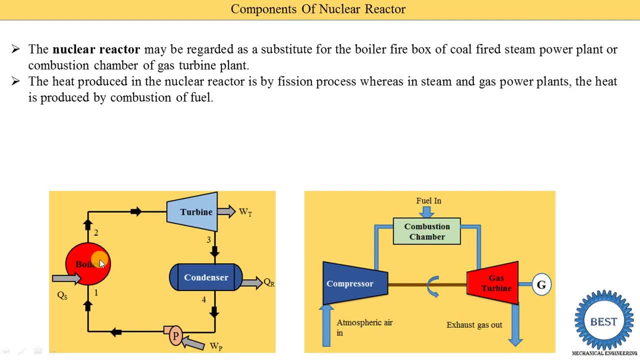 or by combustion of these fuels, the heat is released and this heat is used to heat the working fluids. okay, in a nuclear reactor, the fission process is carried out and due to fission process, the heat is released and this heat is utilized to heat the working fluids. 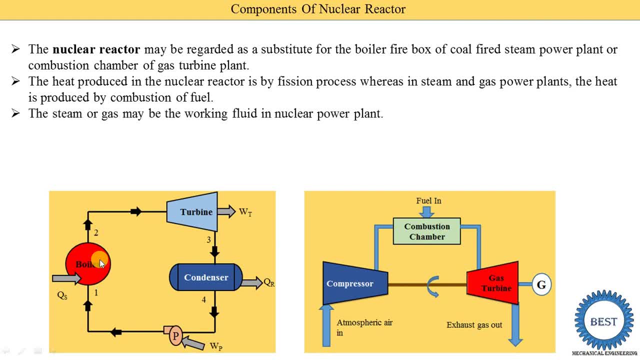 the steam or gas may be the working fluid in a nuclear power plants means, according to the types of the power nuclear power plants, the working field may be streams or working field may be gas. the other cycle of operations and the components require is the same, either as a. 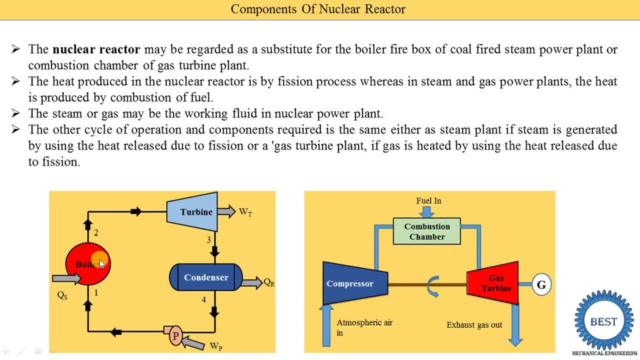 steam plant if the steam is generated. means suppose we generate the steam in a nuclear reactors- okay, then other parts are same. means suppose, instance of the boiler, here we put the nuclear reactors- okay, then the steam is supply into turbine, condenser and pump. okay. and suppose we use the gas as a working fluids, okay, then its other component are same. 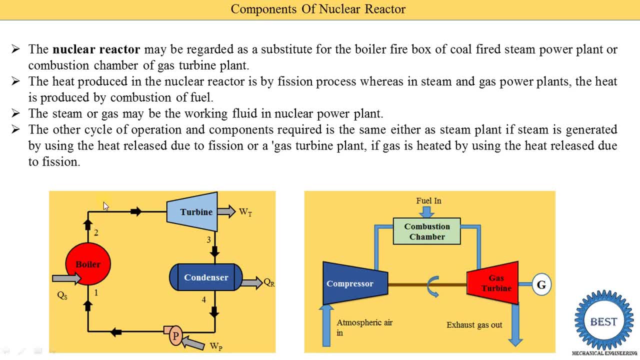 as the gas turbine power plant means, that is, the compressor, is that instance of combustion chamber that is, a reactor is there and after the reactor the hot gas is supplied into these gas turbines and then, after it is passed from heat exchanger or directly supplied there to the exhaust. okay, 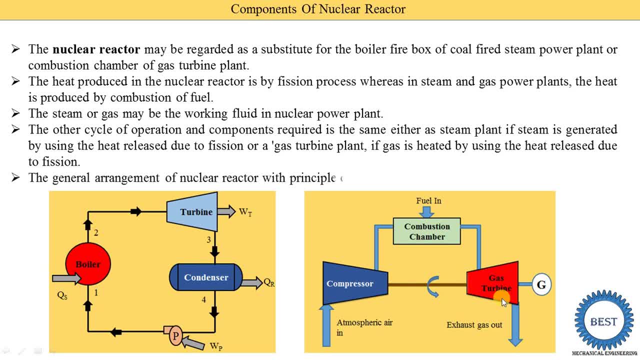 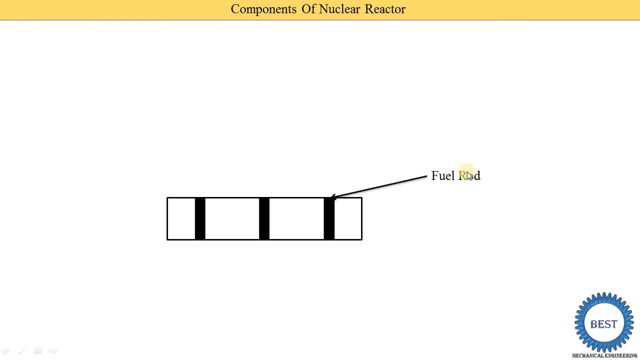 the general arrangements of nuclear reactors with principal component is shown in this. now we understand the basic components by using this animation. here you see, this is the nuclear fuels. okay, so here i mention it is the fuel road, and this fuel road is surrounded by the moderators and this is called as the core of this nuclear react. 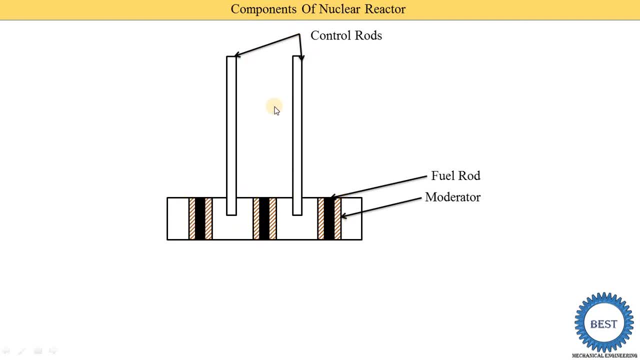 and between this, this, this fuel, the control rods are provided, okay, and this control rod are able to move up and down. then, after this part, is the reflectors, and after the reflectors, that is, the other part is there. it is called as the reactor vessels, and after the reactor vessels, this is the biological. 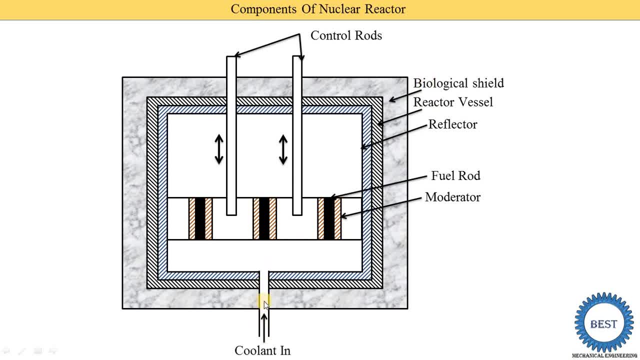 shield are there and from this space coolant is in. coolant means the working fluid is enters and from this side this coolant is out. now we understand all this. component means which type of the fuel is used, which types of the moderator is used. what is the functions of all the components? 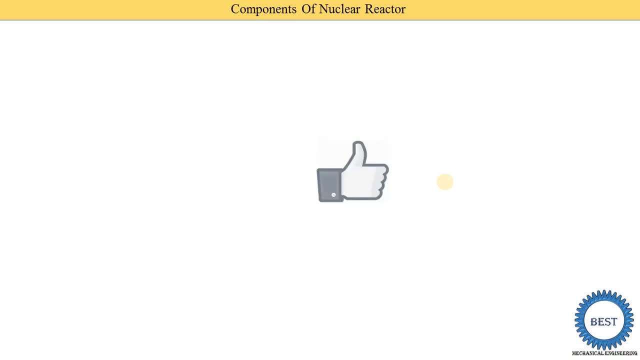 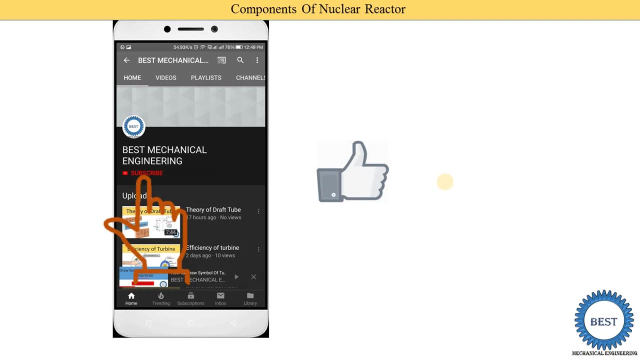 that we understand in this sessions. now, before moving ahead, i request to like the video and subscribe my channels for watching more video related to power plant engineering, as well as the other subject of this, mechanical engineering. for power plant engineering, where is link is provided in descriptions as well as in card? for other subject, i request to visit. 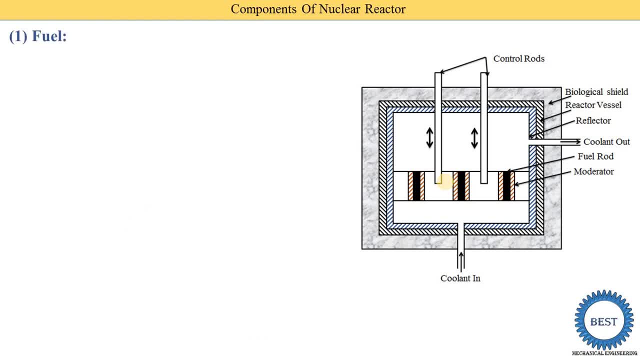 you in the next video. Thank you the playlist. so first component is the fuel. nuclear reactor use. fissionable material means fissionable fuels are used like uranium 235, pu 239 and 92 uranium 233. natural uranium found in the earth crest has 0.71 percent of 92 uranium 235. okay means majority. 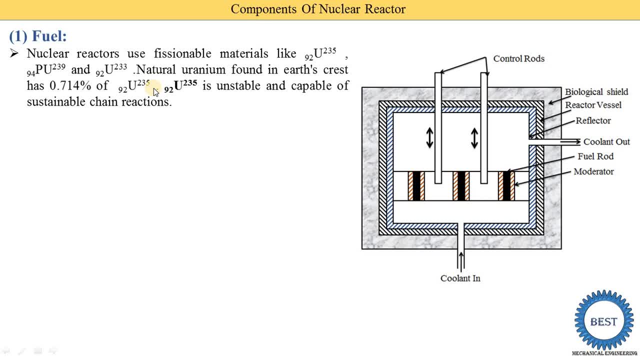 92 uranium 235 is used as fuels and this is uranium means. 92 uranium 235 is unstable and capable of sustainable. chain reaction means are usually names are yet able to understand a chain reactions fuel is said in a very safe like road. here use it is that in the set of 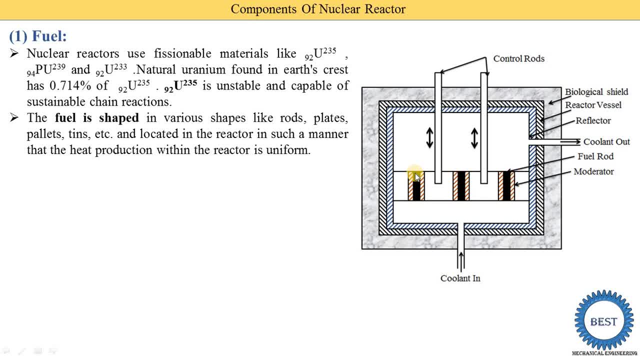 the roads, but we are able to put the fuel in different shape. okay, so we are use the road shape plates, pallet tins, okay, so these are the various. shape is possible and located in the reactor in such a manner that the heat production within the reactor is uniforms means they are arranged such a way that the heat produced is uniform. 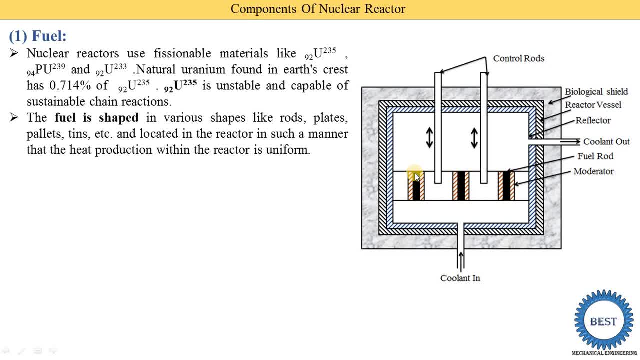 means the same quantity of heat removed from the fuel and means in a reactor the uniform heat productions are there, the fuel elements are designed. it taking into account the heat transfers, corrosions and the structural strains means this fuel element, means fuel shape is designed at that time. they are focused on the three parameters. first is the heat. transfer means the heat. 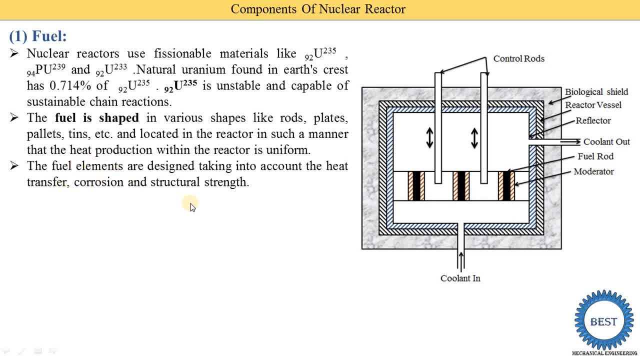 production. second one is the corrosion and the third one is the structural strength. so that is, the two types of the reactor is possible. one is the heterogeneous and another is the homogeneous. okay, so heterogeneous reactor means the fuel is used in a form of road plates and moderators surround the fuel elements. so in this diagram you see that is the first fuel. 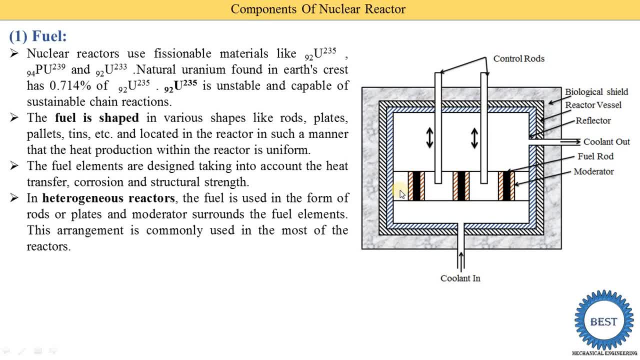 road is there and the fuel road is surrounded by the moderators. okay, so in this diagram we see these heterogeneous reactors. okay, and this arrangement is commonly used in the most of the reactor. second one is the homogeneous reactors. homogeneous means the fuel and moderators are mixed to form a uniform mixer. means fuel and moderator are mixed, then after they 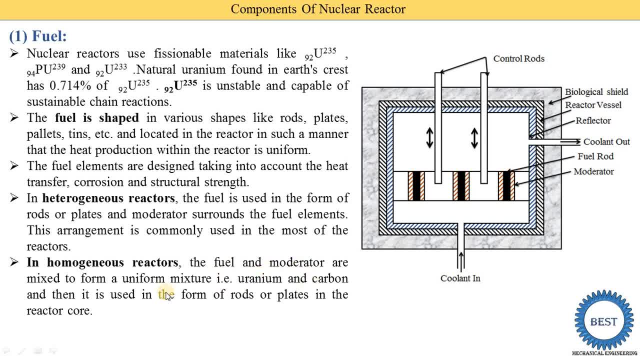 are put in these reactors, so uranium and carbon, and then it is used in the form of roads and plates. in the reactor, code means uraniums and carbon are mixed and by using them, the fuel, roads are created or a plates are created, and then, after they are, 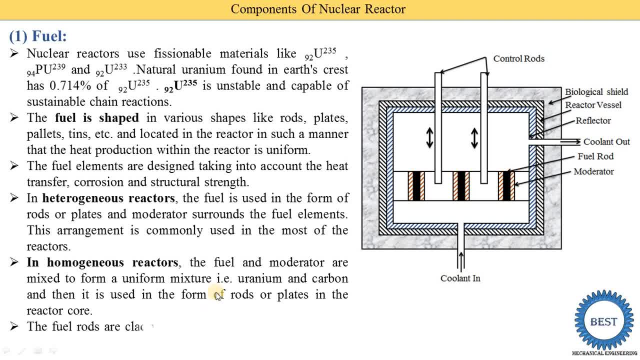 putted in the reactor core, the fuel rod, are clad with stainless steel, zirconium, or by aluminium to prevent oxidation of uranium. is this fuel rod? okay? this black color portion is the fuel rod and they are coated clad means they are coated with the stainless steels or a zirconium or a by. 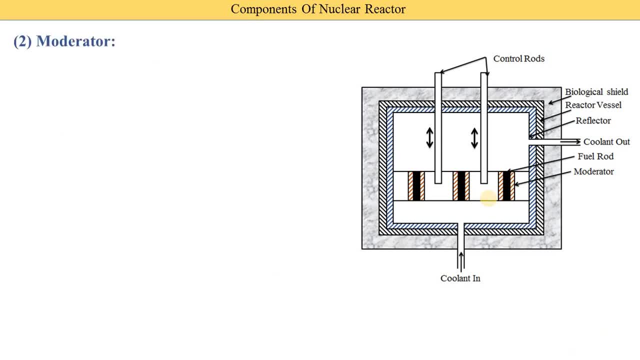 aluminiums to prevent the oxidations of the uraniums. second component is the moderators. it is a material used to slow down the neutrons from high kinetic energy, to slow newton in a fraction of second means. it is used to reduce the velocity of a newton's okay so. 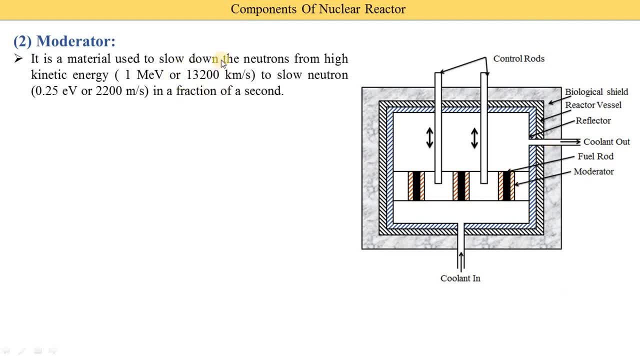 newton component coming out from the fuel have a velocity of 13200 kilometer per second, and it is reduced to 2200 meter per second. okay, so here only this digit is not reduced, but here, you see, the unit is also reduced. that is a kilometer per second to meter per second. so it is a very big change in this. 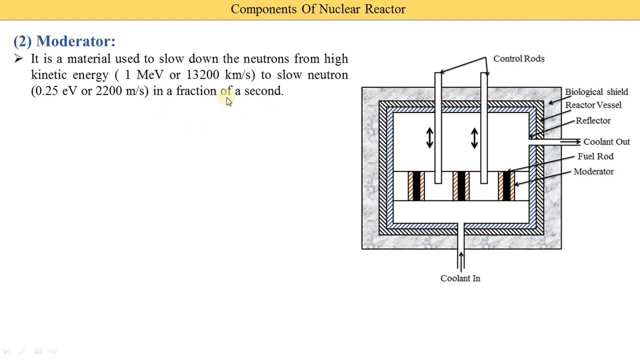 velocity and it is in the within a second, in a fraction of seconds. the function of moderator is to increase the probability of a reactions means increase the probability of chain reactions. the fission chain reaction in the nuclear reactor is maintained due to the slow neutrons when the 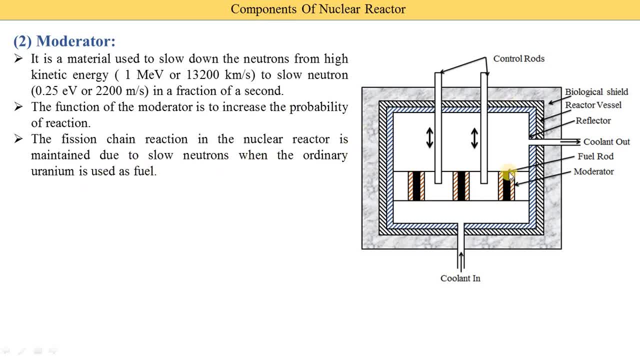 ordinary uranium is used as a fuel. means, when we use the ordinary uranium as a fuels, okay, at that time this chain reaction is continued due to the slow speed of the neutrons. okay, that's why the slow speed of the Newton is important. okay, if suppose the high speed of the Newton is there. 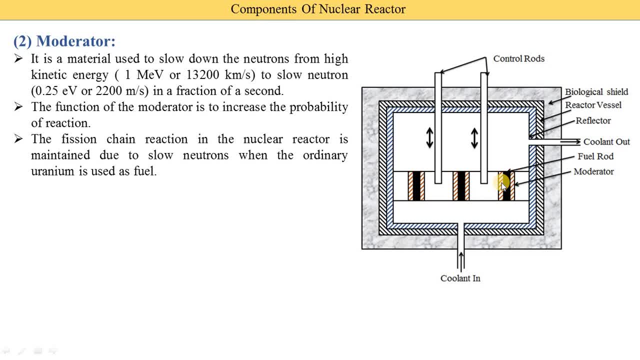 then the chain reactions are not maintained. okay, so for maintaining these chain reactions we need to reduce the Newton speed, and Newton speed is reduced by using this moderators. the moderators are lighter than fuel. various material used for moderators are: first is the ordinary waters, means h2o. second one is the deuterium, or a heavy water. 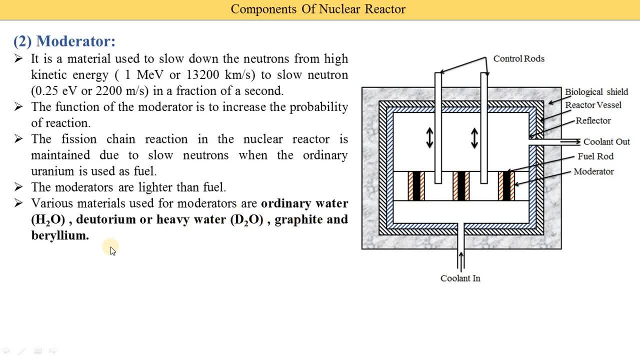 it is denoted as d2o. third, one is graphites and four one is the berylliums. so these are the various four substance that may be used as a moderators. the graphite, heavy water or beryllium can be used as a moderator with natural uranium means when we use the natural uranium as a fuel, at that time we 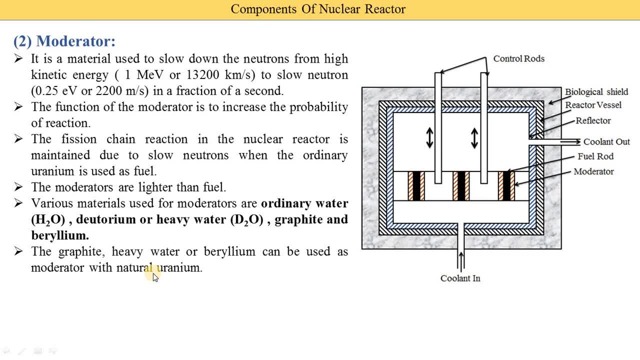 have a three option or a. we have a three options of material for the moderators. first one is graphites, heavy waters and berylliums. the ordinary water means it is a simple water that we drink, that is. the h2o is used as a moderator only with the enriched uraniums. okay, so when we use the enriched 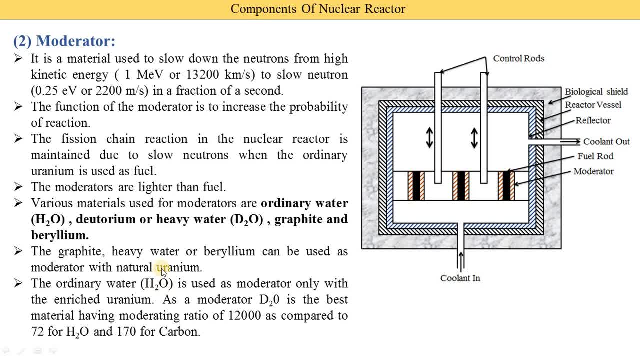 uranium as a fuels. at that time we are able to use the ordinary water as a moderators, as a moderators d2o. d2o means heavy water is the base materials. having a moderating ratio of twelve thousand as to seventy two for h2o or 170 for the carbons, means this is the value of moderating ratio. okay. 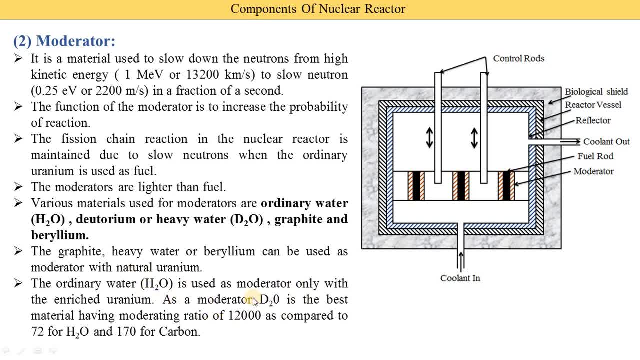 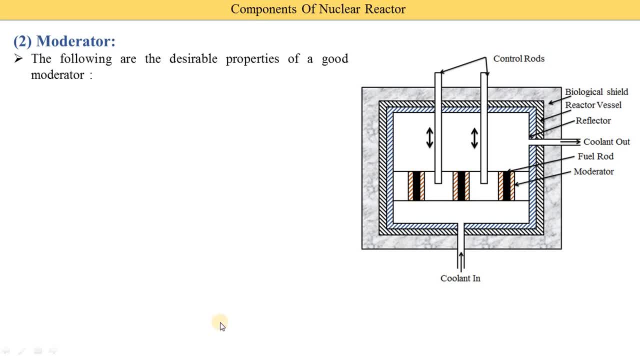 so that is the this h2o- sorry, d2o means heavy water at the base moderators. the following are the disabled properties of a good moderators. first is the moderator must be as light as possible. the slowing down action is more effective. elastic collisions with the light elements means it is light in weight. then they are very efficient. 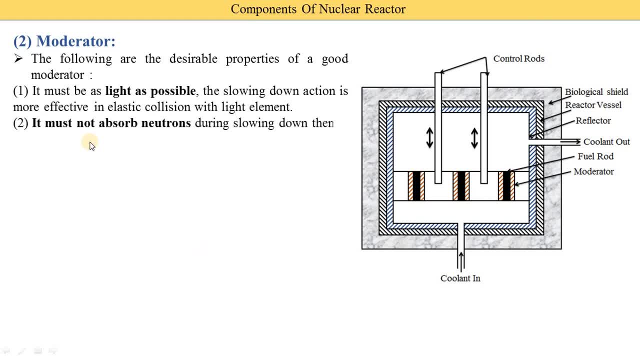 or they are very effective. it must not absorb Newtons during the slowing down them means when these moderators are reduced the speed of the Newtons, at that time they are not able to absorb the Newtons. okay, they are just reduce the speed, they are just reduce the velocity of the Newtons. 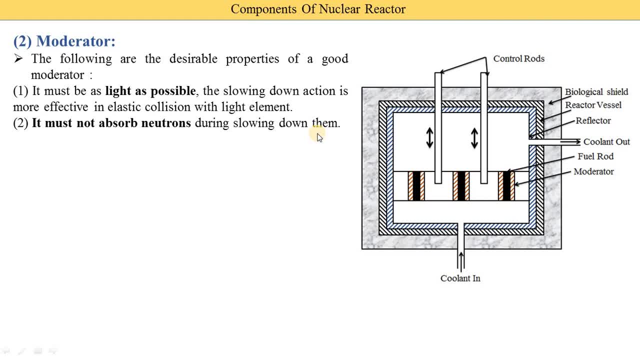 but must not absorb the Newtons. it must be able to work under a high pressures, high temperature with good corrosion resistance means at the high pressure and high temperatures they are good corrosion resistance. it must have high chemical stability as well as its sole is not be decomposed due to the nuclear radiation means they're not react. 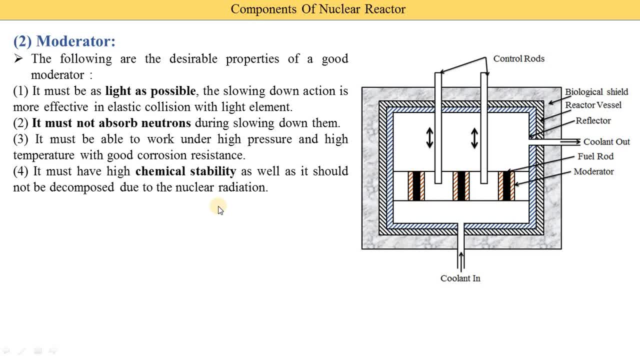 with some chemicals means they are come in the contact with the fuels, they are come with the contact with the coolant. okay, at that time they are chemically stable. they are not change this chemical formula. it is called as the chemical stabilities. now the third component is the. 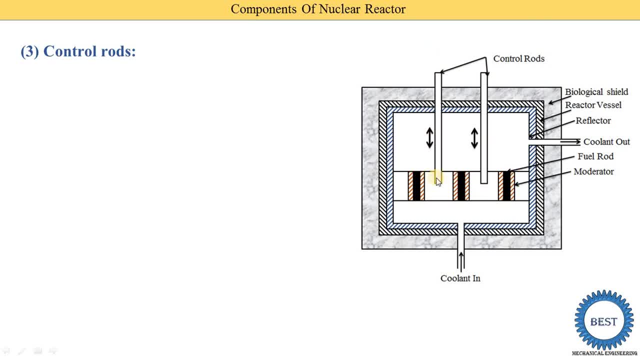 control roads. so in this diagram here you see this control road are putted between these different fuel roads. okay, so what is the functions of the control road? why these control roads are requiring these nuclear reactors. the control system control the rate of energy generated. so from the name we can understand control roads means they are controlled rate of energy. 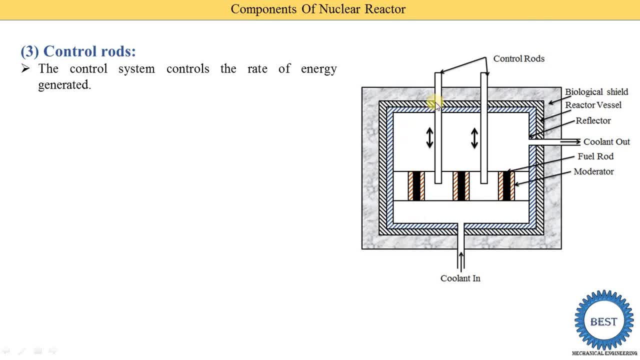 generated means. when we move these control road up and down, we can start the chain reactions, we can increase the chain reaction, we can reduce the chain reaction or even we can stop the chain reaction. that's why its name is given: the Control road. so what they control? 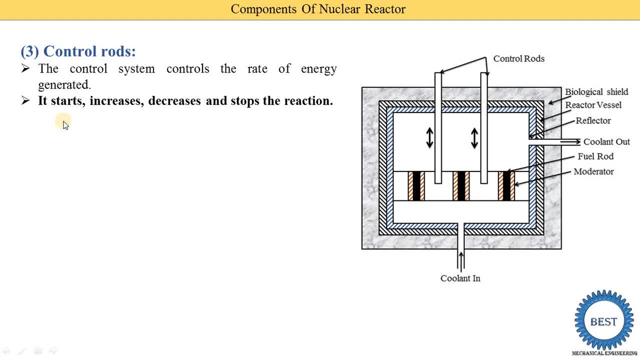 control the rate of energy generated means it start, increase, decrease and stop the chain reactions. that why its name is given the control roads. this road may be shaped like the fuel roads themselves and are interspread throughout this reactor core. now, what is the reactor core? this combination of the moderators and the fuel roads. it is called as the reactor cores. okay, and here, 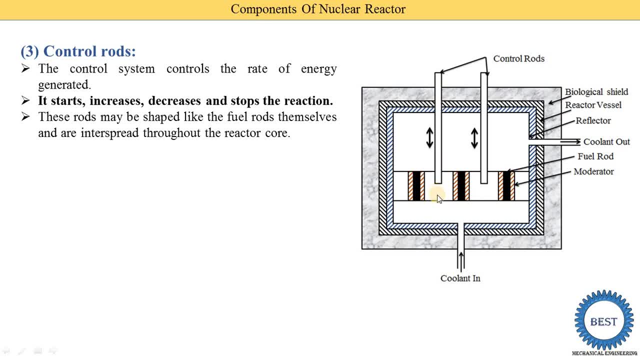 you see this: the fuel roads are insert in a reactor core means they are move up and down in this reactor core. means when we fully remove that, at that time this feed of the chain reaction are higher. when these control roads are move down, means they are inserts in a reactor core at that. 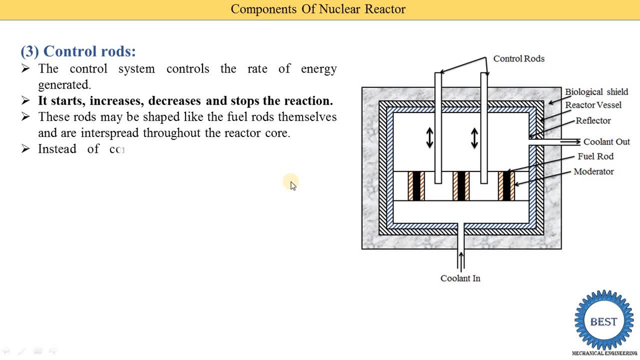 time this chain reactions are stop. instance of containing fuel: they contain newton absorbers such as the boron, cadmium and indium, means these are the material used as a control road. they have high newton absorption cross section means they are absorbs the newtons. that's why they are able to control. 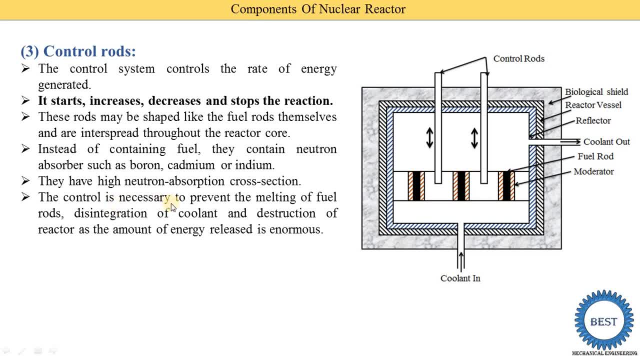 the chain reactions. the control is necessary to prevent the melting of fuel, roads, disintegrations of coolant and destructions of the reactor. as the amount of energy releases and romeos okay means this, control of the chain reactions are very important to avoid this melting of fuels, disintegration of the coolants. 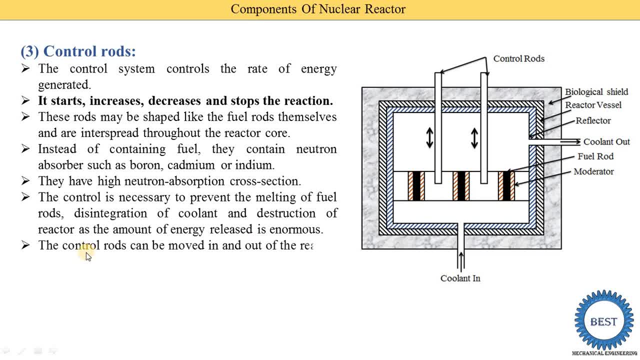 and there are other reasons. the control role can be moved in and out of the reactors core assembly either automatically or manually means these control roads are move up and down. here we draw already the arrow. so these moving process are either manually or either automatically means they are operated by using this robot, or they are operated by human. 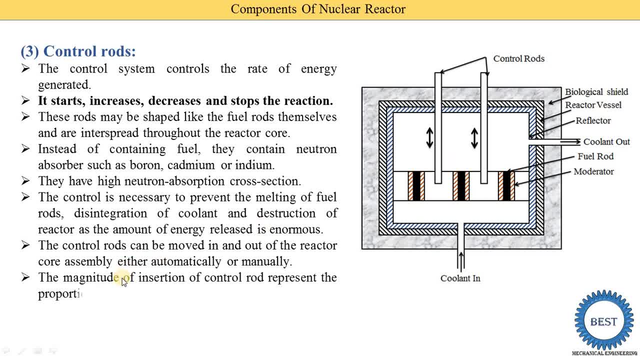 The magnitude of insertion of control road represent. the proposed net absorption of Newtons means we insert this control droid in a reactor core, then these reactions are stops. okay, when we remove from this reactor core, then the chain reaction start or they are increase. now forth component is the coolant. 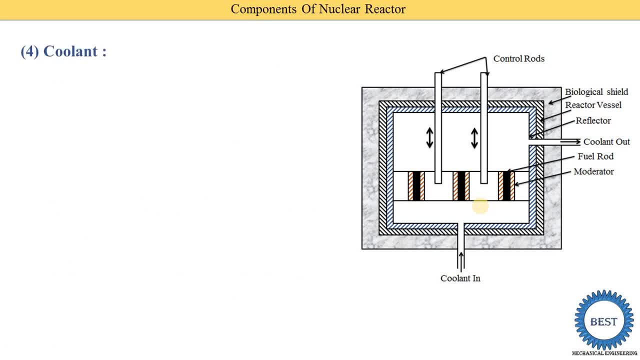 is the coolant. we can also say it is the working substance of the nuclear power plants. so from the name we can understand what is the functions of the coolant. coolant is absorb the heat from the nuclear fuels. so main purpose of the coolant in the reactor is to transfer the heat produce in 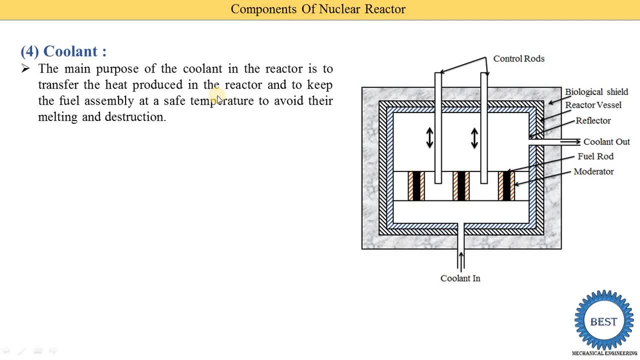 the reactor and keep the fuel assembly at a safe temperatures to avoid their melting and destructions. means when we pass the coolant and the course, suppose we can see that this is the working fluids. okay, so once we supply this ordinary waters, then water is absorbed, this heat energy from the fuel and the fuel temperature is reduced and this water is converted into the. 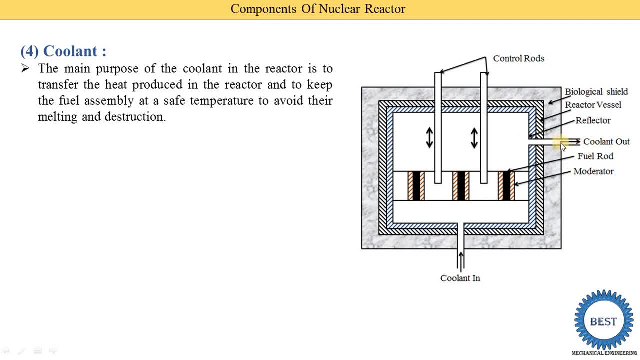 steam. okay, so here from this place this coolant is out means suppose the steam is coming out. then steam is to supply to the turbines or there is a one heat exchanger is put in between. okay, that is a different possibilities are that, according to these types, the same heat carry by the coolant is used in the heat exchanger for further utilizations in the 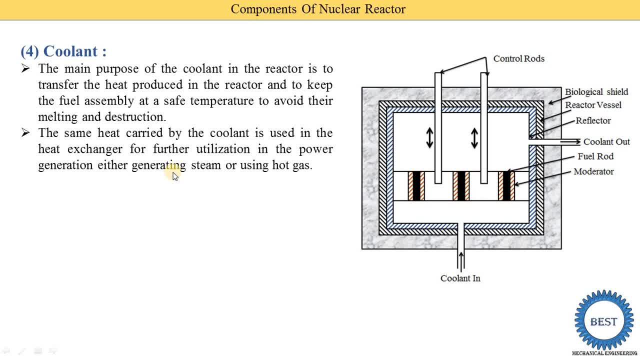 power generations, either generating steams or using the hot gas, means we can supply this gas. then the gas temperature is increased. suppose we supply this water and it is converted in steam, then after one heat exchanger is put it and from this heat exchanger the from the other pipes, the, 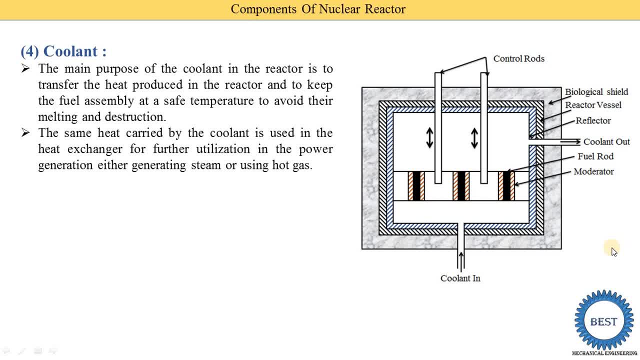 water is entered and this water is converted into the steam means for the safety purpose. to avoid these radiations we can put this one more heat exchangers. the coolant use shall have high specific heat to reduce its mass flow rate means. suppose we required a less mass flow rate? then we can use the material which have a high 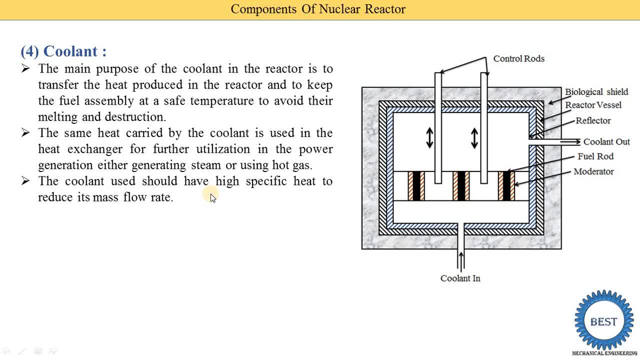 specific heat means high specific heat coolant are able to absorb. the more heat who can they absorb? the more heat then they are converting to the steams, or they absorb. the more heat means its temperature are more increase. it shall not absorb neutrons and it must be non-corrosive, non-toxic, non-oxidizing, with high chemical stability. means: 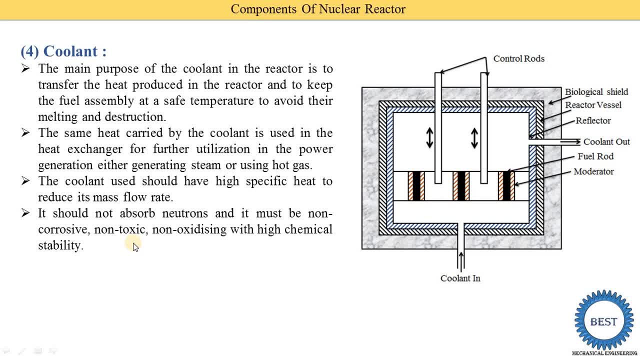 coolant not absorb neutrons. okay means we need to use such a such a types of the coolant. they are not absorb the neutrons. okay. they are non-corrosive, non-toxic, non-oxidizing, with high chemical stabilities. Now, what are the various material used as a coolant? 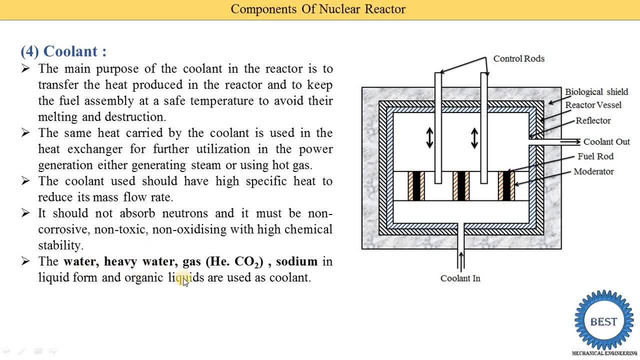 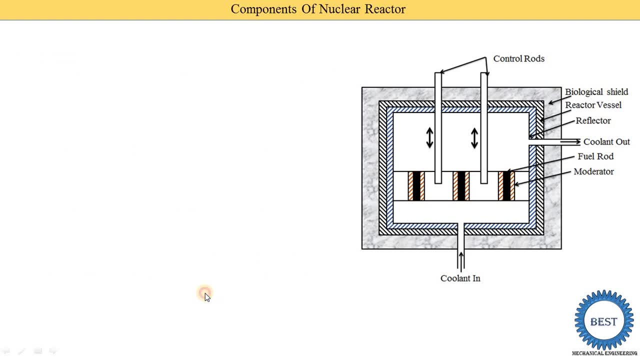 First one is the water, heavy waters. so these are the liquid. suppose we can use the gas as a gas. we can use the Helium, or CO2 means carbon dioxide. another are the sodium in a liquid form and organic liquid are used as a coolant. So these are the very important. 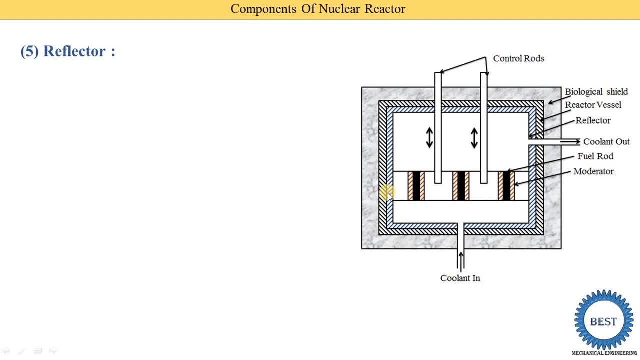 components. then after that is here, you see, these 3 components are used as a valves for the different purpose. This is the reflectors, reactor vessel cells and biological cells, for the word you can already understand. reflector are used to reflect the Newton's okay, so it is important to conserve the Newton as 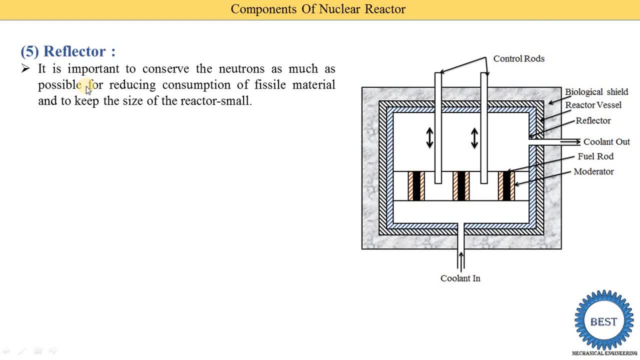 much as possible for reducing consumption of feasible materials and keep the size of the reactor smalls means they are used to reflect the Newton's, and by these reflectors we can reduce the size of the reactors. so this is possible by surrounding the reactor core. what is the meaning of reactor core? 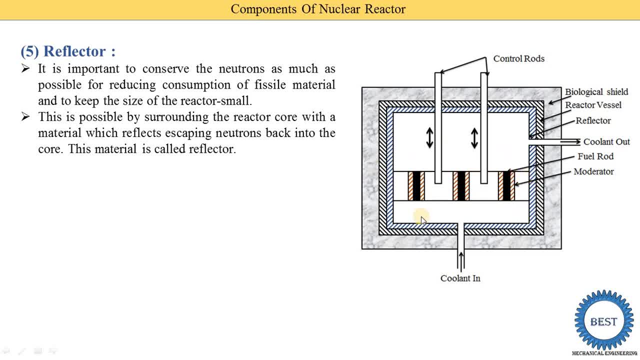 reactor core means this fuel roads and a moderator part is called as the reactor core. so this is possible by surrounding this reactor code with a material which reflect escaping Newton's back into the core and these material is called as the reflector means sometimes this new, new. 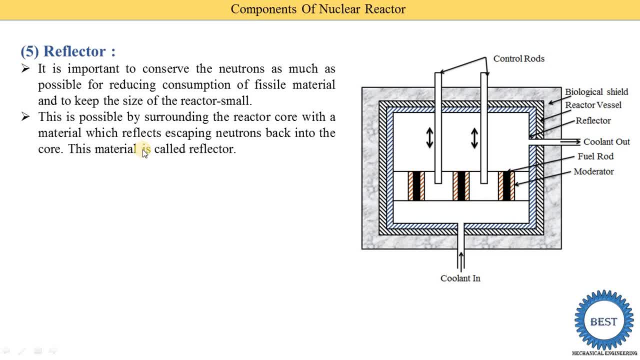 Newtons are escaping from the chain reactions. Okay, So these Newtons are come into contact with the reflectors and the reflector is again span the Newtons or again return these Newtons into a chain reactions or in a this core of the reactors. The required properties of a good 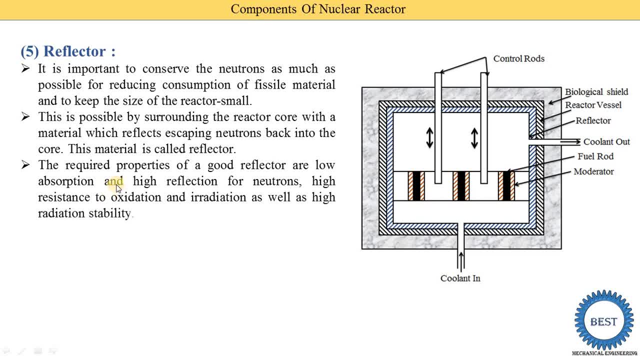 reflectors are: low absorption and high reflections for the Newtons. high resistance to oxidations and irradiation, as well as the high radiation stabilities, Means reflector not absorb the Newtons. They just only reflect the Newtons, Means high reflections for the Newtons are required. 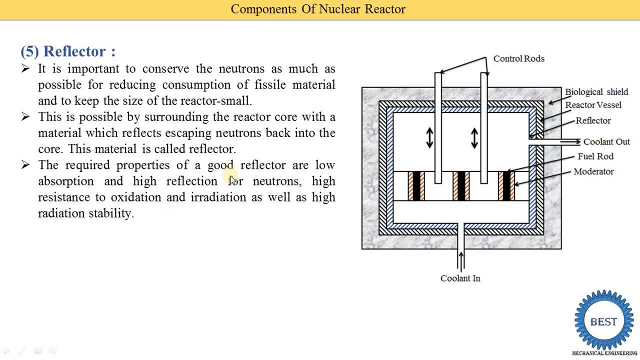 Then high resistance of oxidation is required and irradiations as well as the high radiation stabilities. Okay, The material used for the moderator are also used for the reflectors, like as the H2O, D2O and the carbon. It is necessary to provide some matter of cooling the reflector as it. 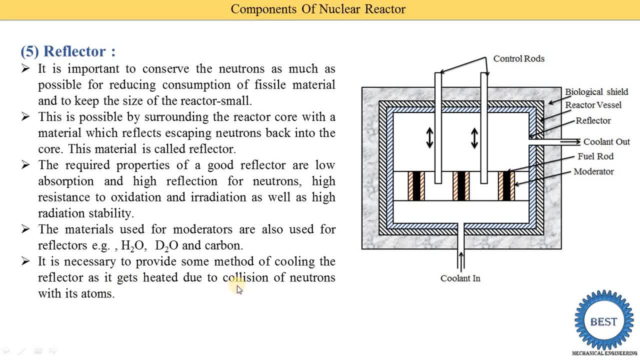 gets heated due to the collisions of Newtons with heat atoms. So when these Newtons are strike with these reflectors, at that time this temperature of the reflectors are increased. So we need to provide one cooling mechanism. means cooling of these reflectors. surface are required, So we need to provide cooling of the reflectors. 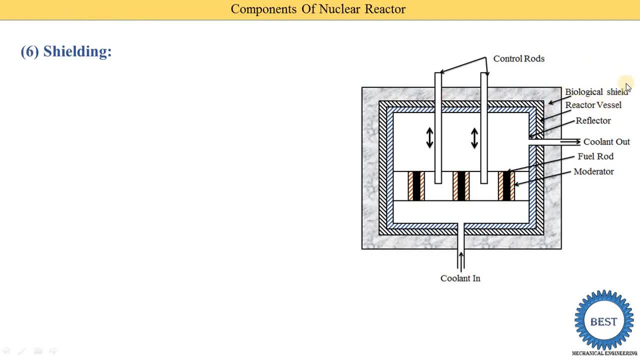 Next component is the shielding. So here you can see that is the biological shield word is mentioned. Okay, So shielding the radioactive zone in the reactor from possible radiation hazardous is essential to protect the human life from harmful effect. Means we know that the nuclear materials are removed the various radiation, So it is called as the nuclear material. 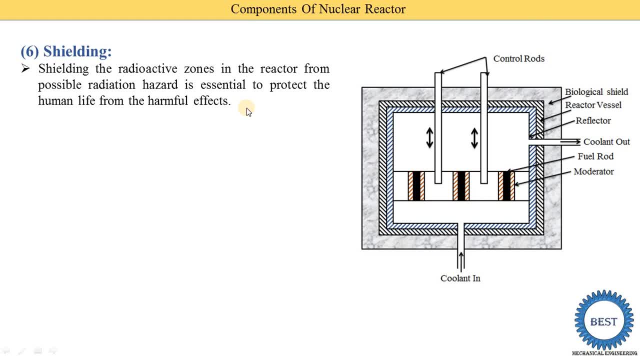 The radioactive materials. Okay, So these radioactive material is stopped by using this biological shields. So common radiations from the reactors are alpha ray, beta ray, gamma ray and the fast Newtons, And we know that these alpha ray, beta and gamma rays are harmful to our 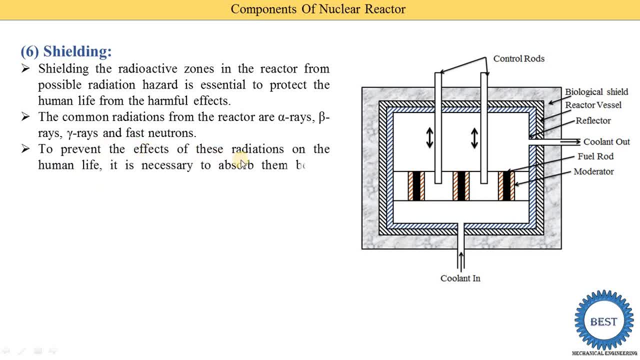 human body. To prevent the effect of these radiations on the human life, it is necessary to absorb them before emitting to the atmosphere, Means we need to absorb these radioactive materials. Okay, And for absorbing these radioactive material that shieldings are provided and it is called as the biological shield, And 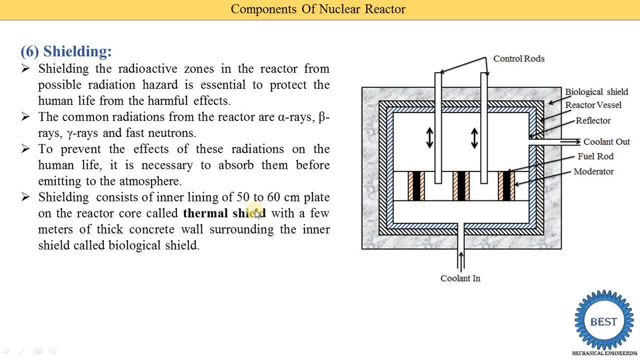 the shieldings is consist of inner lining of 50 to 60 centimeter of plate on the reactor core- reactor core, called as the thermal shield- with a few meter of thin concrete wall surrounding This inner seal, called as the biological seal. Means this: biological seals are combination. 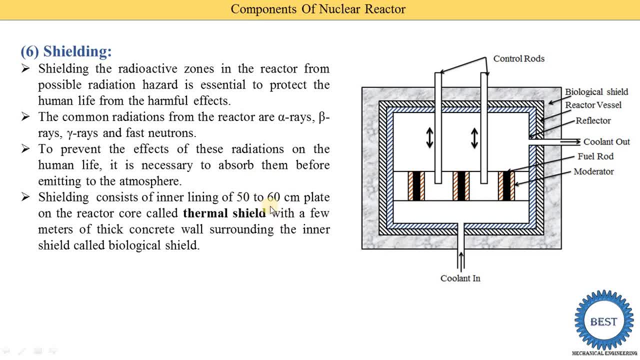 of the two part. First part is the steel plates are used, that is, the thickness is the 50 to 60 centimeters. and then are the concrete walls are there, The lining of steel plate absorb these energies and become heated But prevent this adjacent wall of the reactor vessel from. 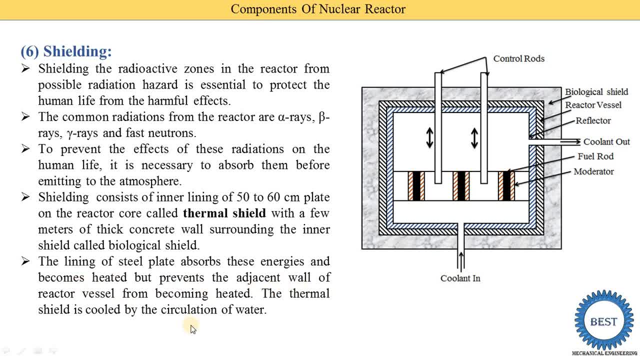 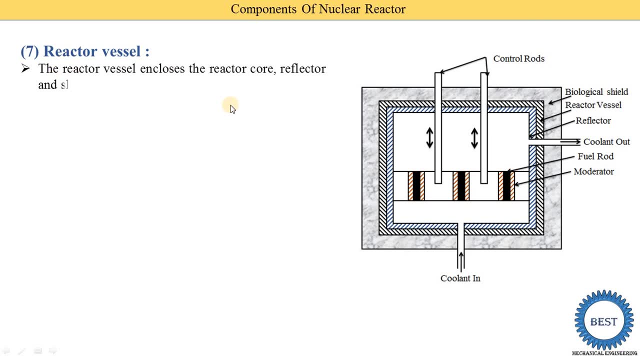 becoming heated And this thermal seal is cooled by circulations of waters. Okay, Thermal seals are heated and then its temperature is lowers by using the circulations of water. And the last part is the reactor vessels. The reactor vessel enclose the reactor core. 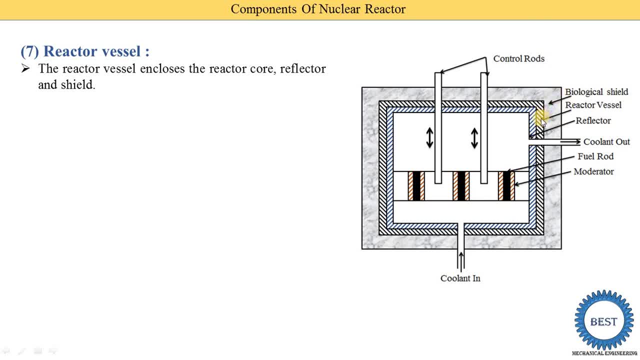 Means here. you see, at the center parts, these reflectors and the reactor vessels are there. Okay, So this is the reactor vessel. So what is the functions? The reactor vessel is enclosed, the reactor core reflectors and the shield. It also provides a 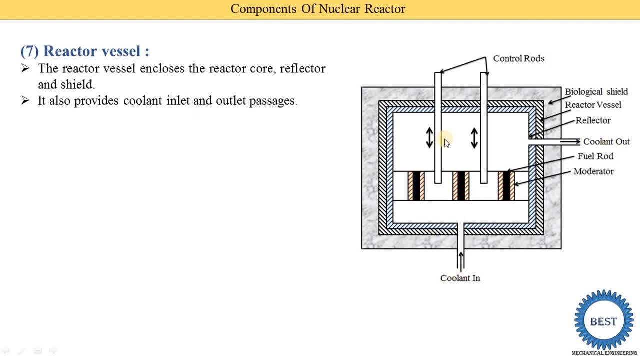 coolant inlet and outlet passage. Here you see this coolant inlet and outlet passage are there. The reactor vessel has to withstand the pressure at 200 bar or above. The reactor core means fuel and the moderator assembly is generally placed at the bottom of the vessel. 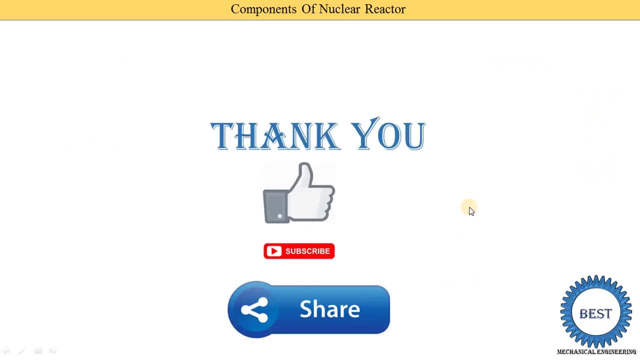 So here you see, at the bottom of this vessel we are putting this reactor core. Okay, So here we complete these various components of the nuclear reactors. If you learn something, then like the video, subscribe my channel and share with your friends.